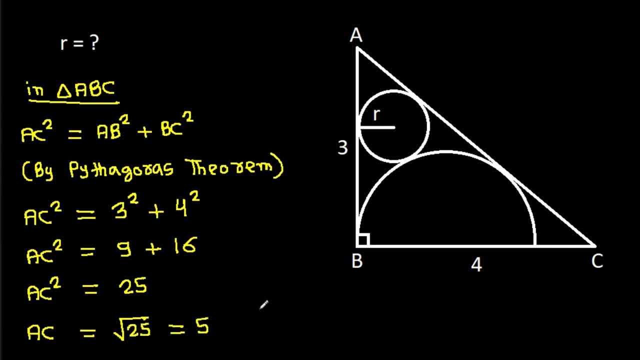 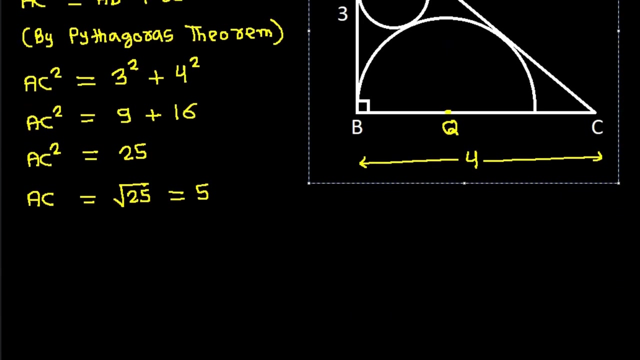 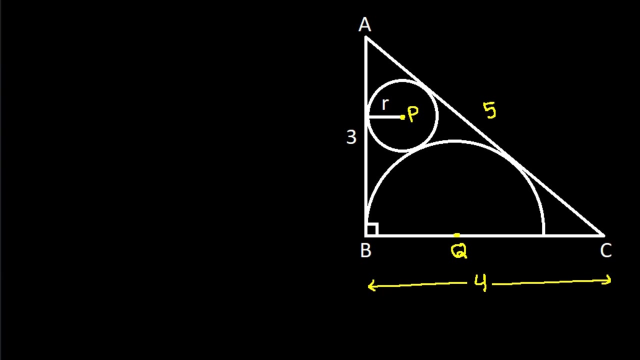 25, that will be 5.. So AC, it is 5.. And now suppose the center of the circle is P, And suppose the center of the semicircle is Q, And we have BC is 4.. And now in any circle, from any point, P, if we make two tangent on the circle. 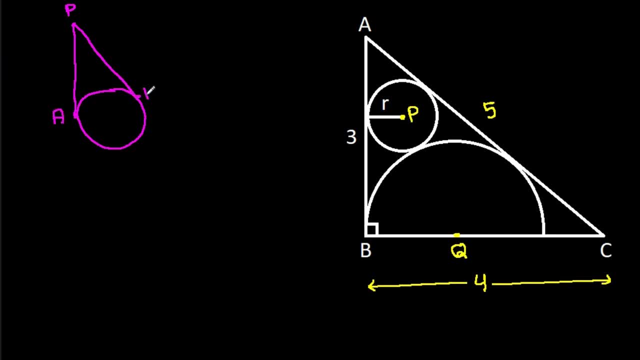 suppose this point is A and this point is B, then PA, it will be equal to PB. And suppose the center of the circle is O, then AO, it will be equal to BO. that will be radius And PO is common. That means the triangle. 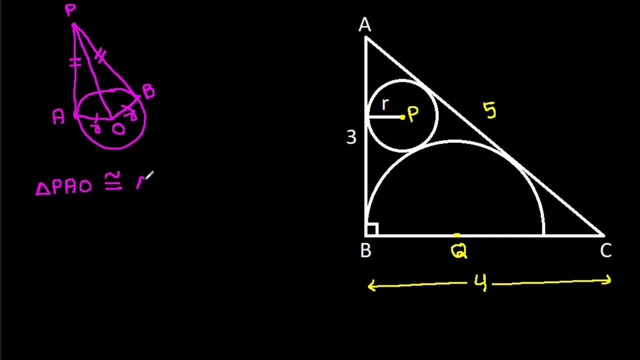 will Entonces el arc radians NY P A, O. It will be congruent to my angle RO and HO, Hence angle APO. it will be equal to AO. And here if we join AP and AO, So PAO it will be congruent to AO, that will equal angle该 AO. 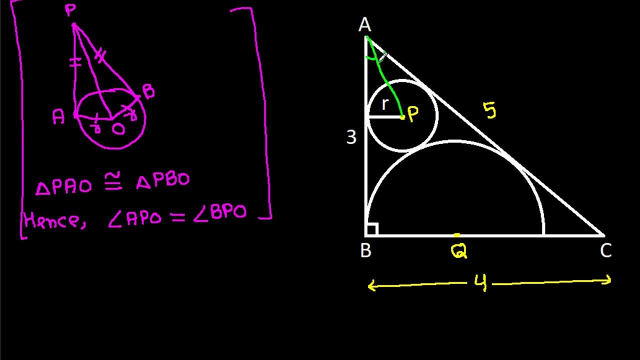 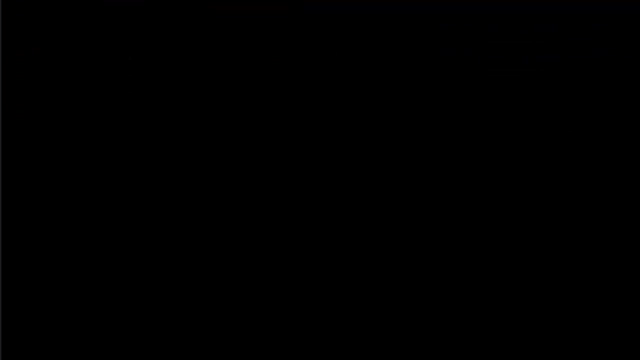 then these two angles, they will be equal. suppose theta and also aq, it will be angle bisector of a, ap and aq. they will be angle bisector of a, so aq, it will pass through p, and now in any triangle- a, b, c, if ad is angle bisector. 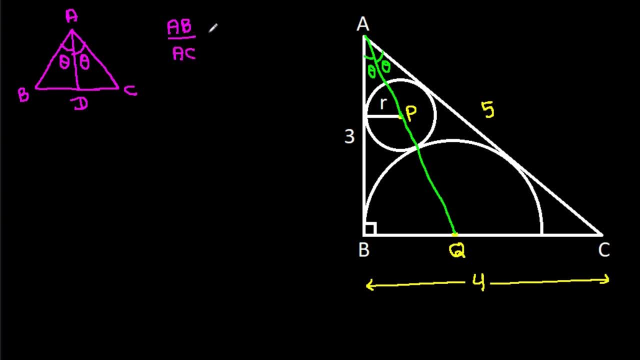 then ab over ac it will be equal to bd over cd. and here in triangle a b c it is a b c, aq is angle bisector and ab is 3, ac is 5, and suppose bq is capital r, then cq it will be 4 minus capital r. 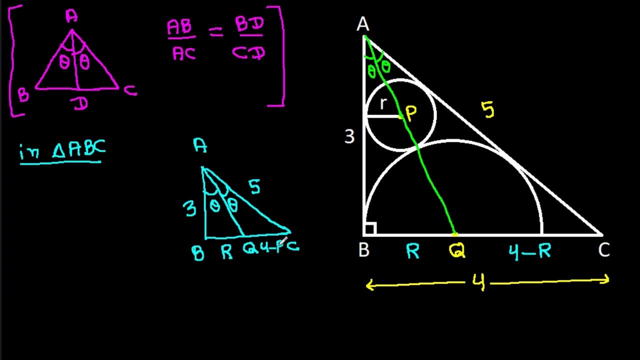 bq is r and cq is 4 minus r and a, b over ac, it will be equal to b, q over c q and ab is 3 over ac is 5. it will be equal to bq is r over cq is 4 minus r, and if we cross multiple i, then twelve minus three are. it will be equal to a, b, c. it will be equal to two less than two. 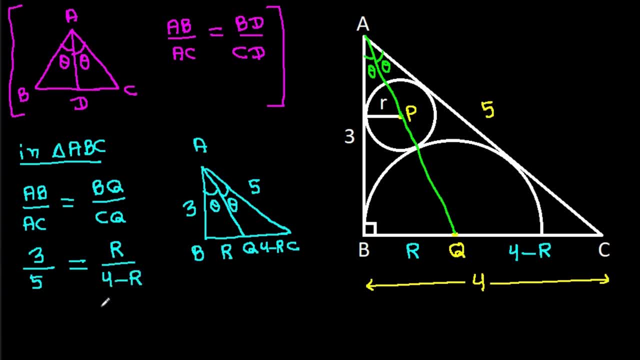 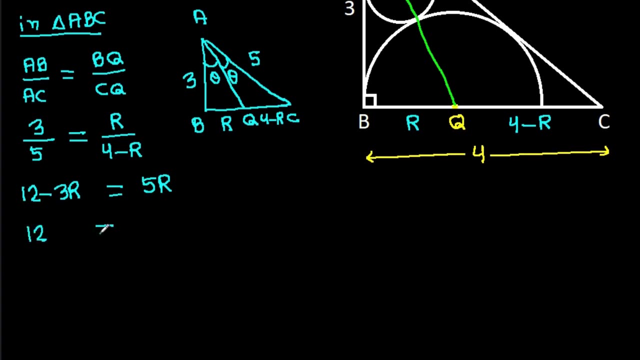 a and c, q equal to a, b, c is equal to b, q over c q, and if we cross everything, then this is 3.. the first time we use this number is 3, and then the second power is 5.. be 5r and 12, it will be 8r, so r it will be 12 over 8. that will be 3 over 2, so we get R is 3 over 2. 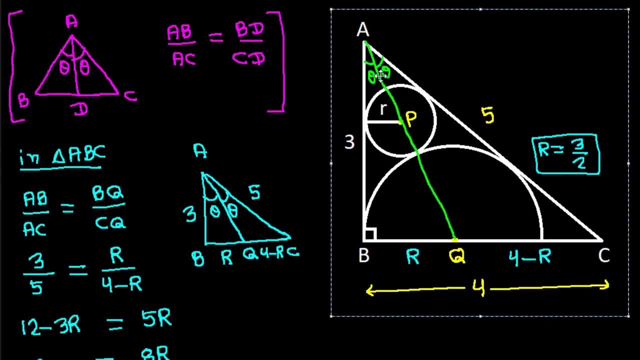 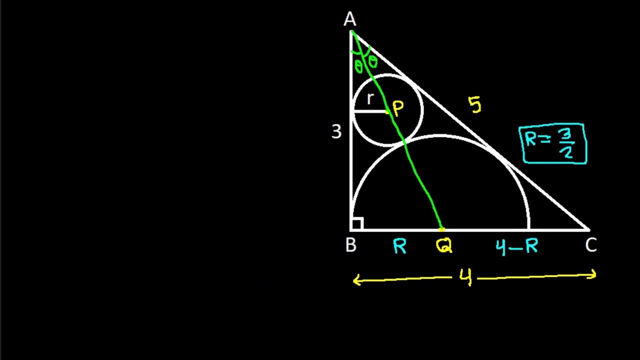 and now inter angle a, b, q, a q square, it will be a b square plus b- q a square by Pythagoras theorem. and a- q a square, it is equal to a. b is 3 a square plus b. q is capital r a square and a q a square, it is 3 a square plus capital r. it is 3 over 2 a square. 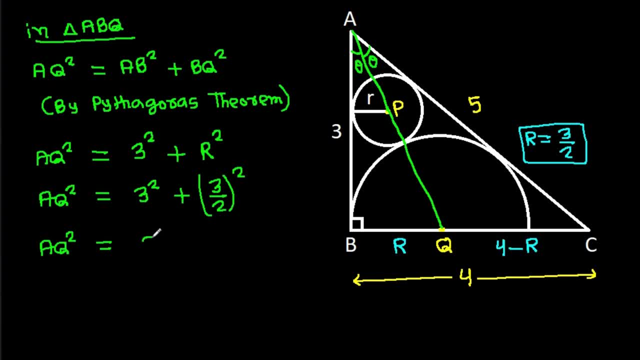 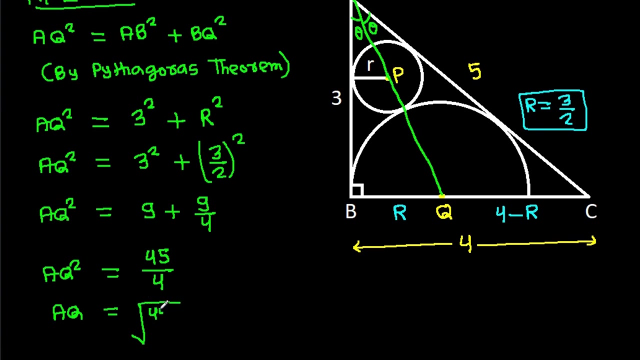 and a q a square, it is 9 plus 9 over 4. and a q a square, it will be 36 plus 9. that will be 45 over 4. so a q, it will be root under 45 over 4, that will be 3 root 5 over 4. and a q a square, it is 9 plus 9 over 4. 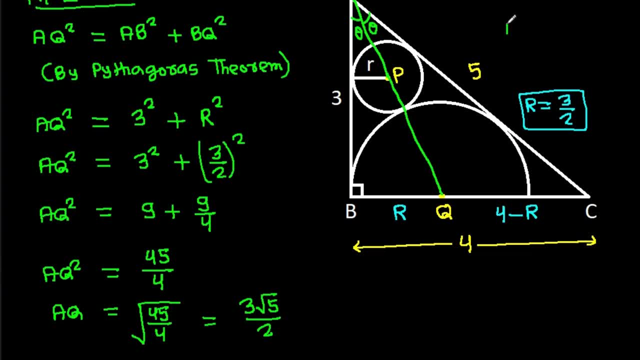 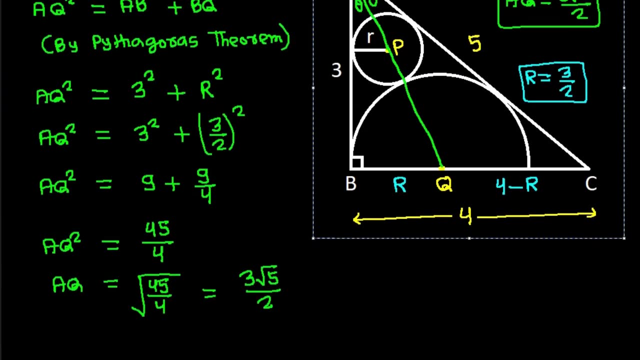 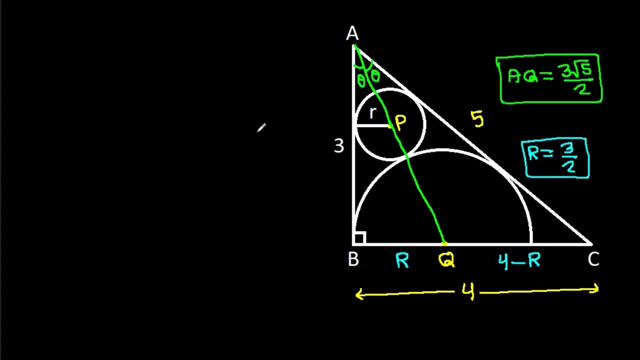 one is 4, this is 4 root 5 over 5 over 2. so we get a- q is 3 root 5 over 2. now we know that in any circle, radius and tangent, they are perpendicular to each other. so this angle, it will be 90 degree, and suppose this point is M and we have a B is 3 and 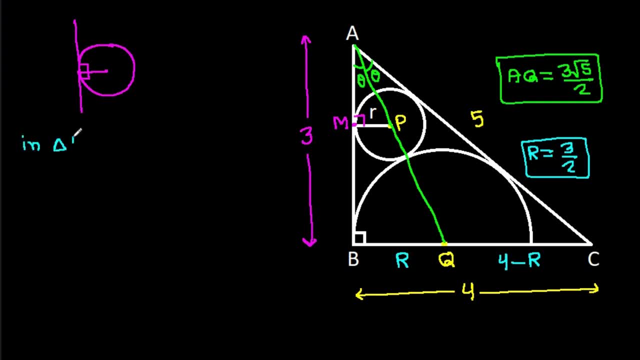 now inter angle AMP and triangle aB, q. sine theta it will be PM over app and sine theta it will be also equal to B, Q over Vielen Triangles in sinus' angle aq and Pm. it is a small r over ap. it is equal to bq. it is capital R over aq. it. 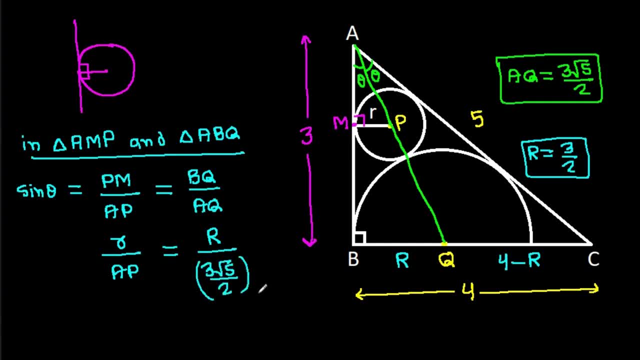 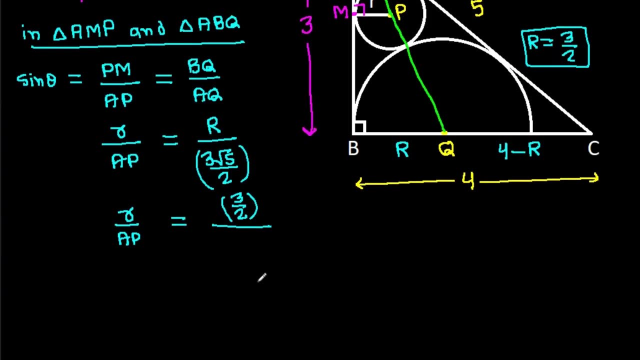 is 3, root 5, over 2, and a small r over ap. it is equal to and capital R. it is 3 over 2, over 3, root 5, over 2, and 3 over 2, will get cancelled. 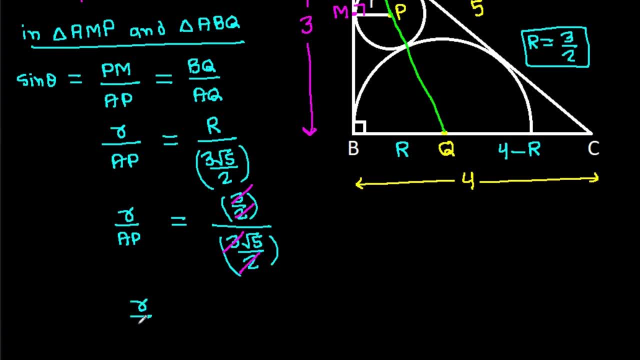 And so R over ap. it is 1 over root 5, so ap it will be root 5 times a small r. we get ap is root 5 times a small r, And and and and. 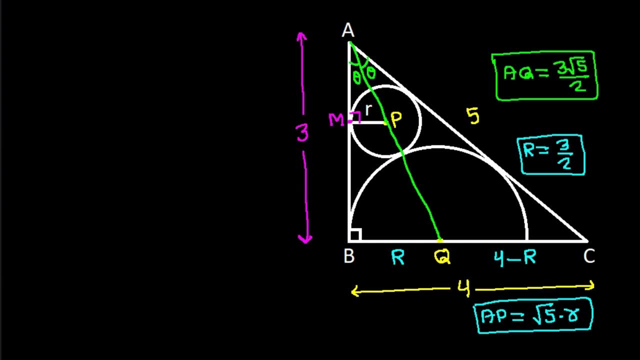 and Now aq, it will be equal. to suppose this point is s, then aq, it will be ap plus ps plus sq and ps it will be a small r and sq it will be capital R and aq it is 3 root 5 over 2, it is equal to. 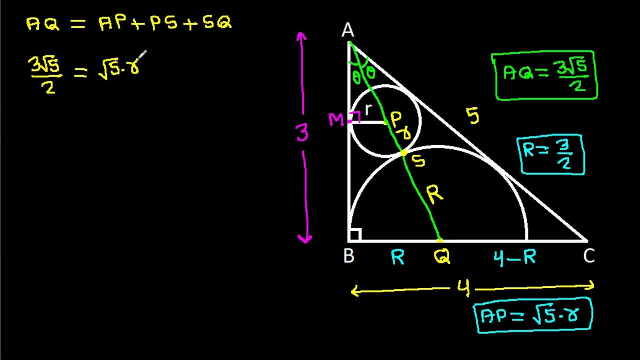 ap. it is root 5 times small r plus ps is a small r plus sq is capital R and 3 root 5 over 2. it is equal to root 5 plus 1 times a small r plus capital R. it is 3 over 2. 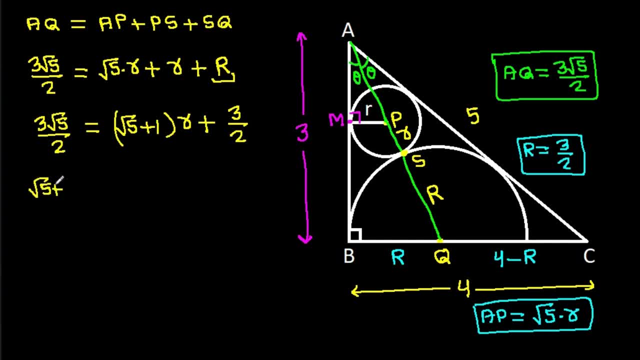 so root 5 plus 1 times a small r, it will be 3. root 5 over 2 minus 3 over 2. and root 5 plus 1 times r, it is 3 over 2 times root 5 minus 1, so r it will be 3 over 2. 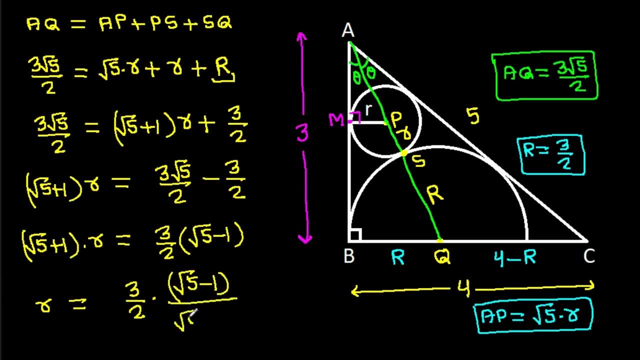 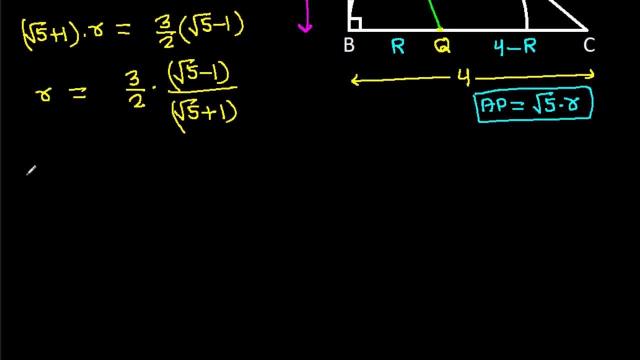 times root 5 minus 1 over root 5 minus 1 and r, it is 3 over 2 times root 5 minus 1 over root 5 plus 1. and if we multiply it with root 5 minus 1 over root 5 minus 1, 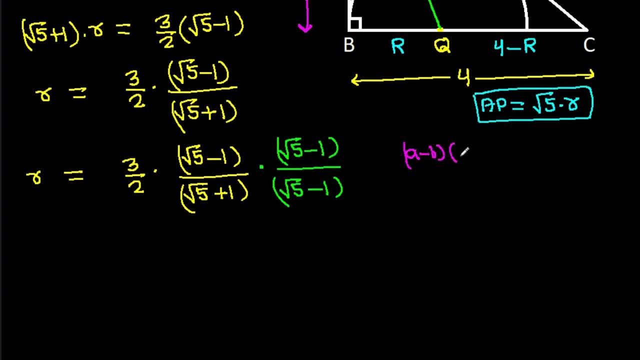 and we know that a minus b times a minus b, it is a minus b a square. that will be a square plus b square minus 2ab. and a plus b times a minus b, it is a square minus b square. so r it will be 3 over 2 times and root 5 minus one times root 5 minus one.